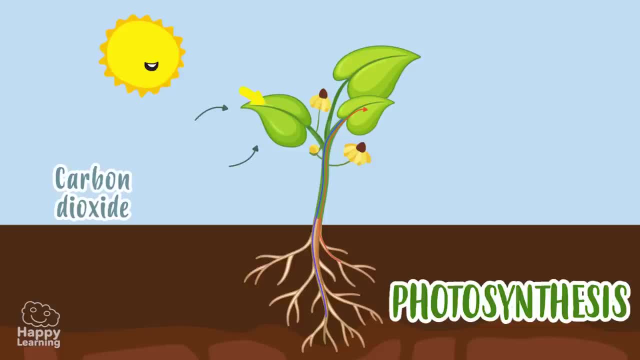 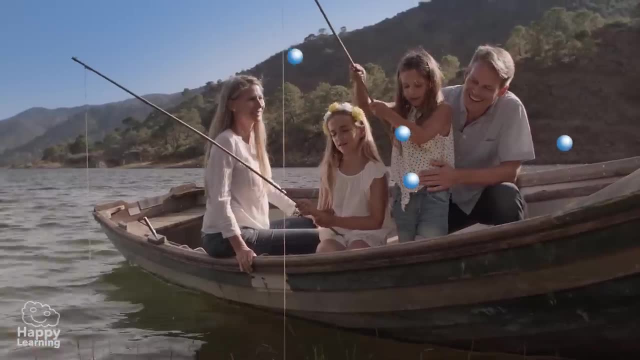 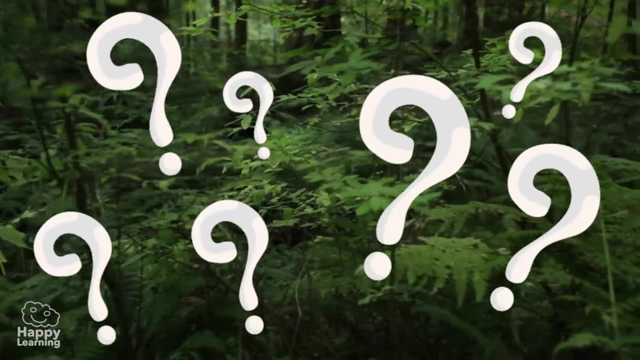 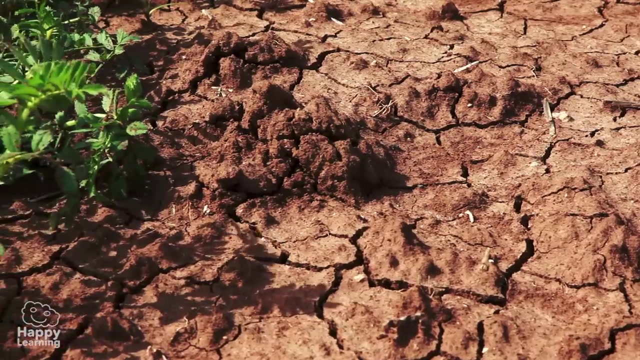 plants, but for all living things too, because in that process they release oxygen into the world, and without oxygen, none of us would be here today watching this video. our plants- important or what? plants- were one of the first forms of life that appeared on earth, thanks to their capacity not to depend on other living creatures to 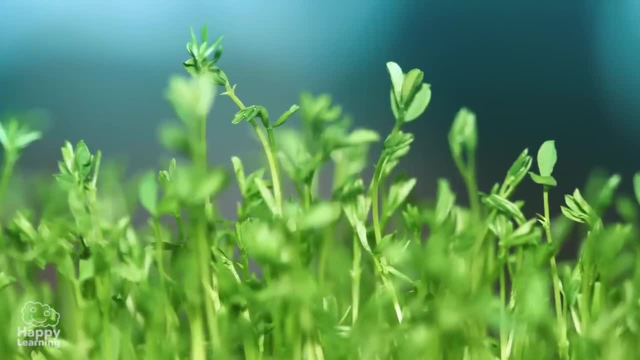 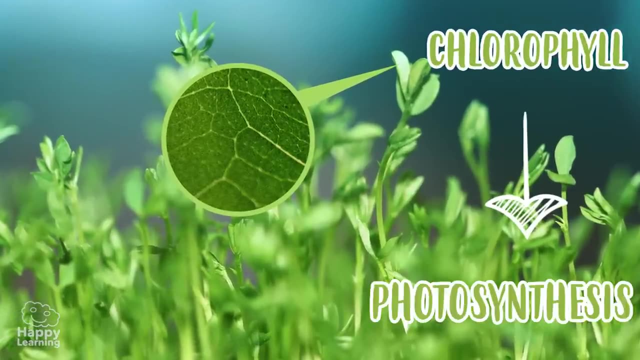 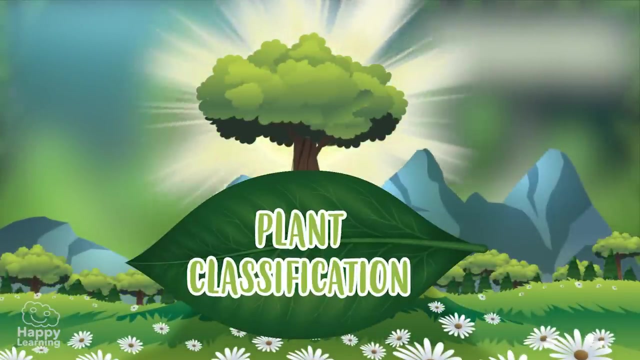 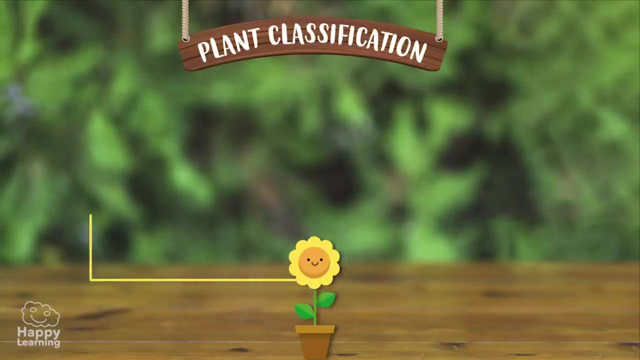 survive. their most predominant color is green and this color is called chlorophyll, an essential substance to perform photosynthesis plant classification. plant classification is an essential substance to perform photosynthesis plant classification. as we said, there are many types of plants and we can classify them in four large groups to get to, 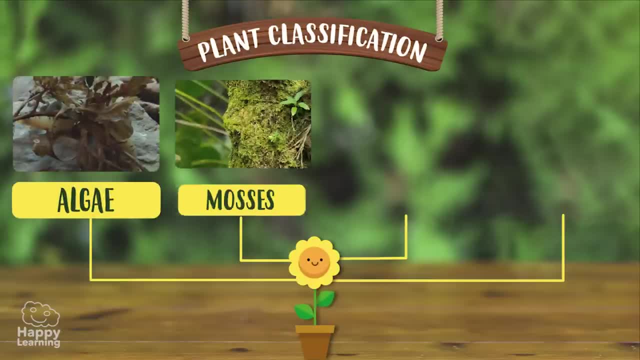 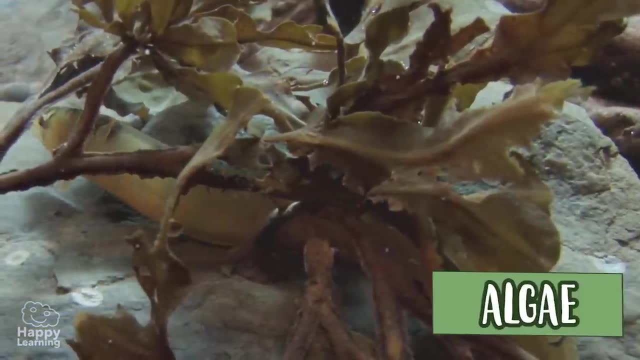 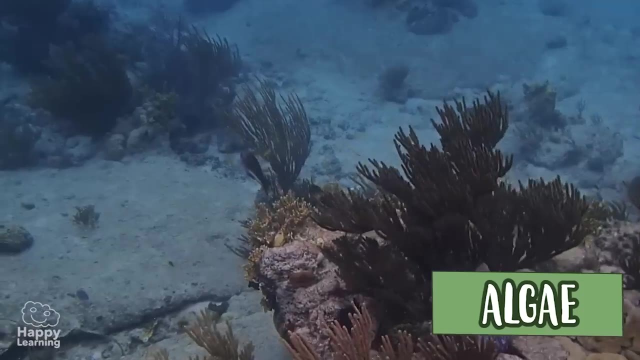 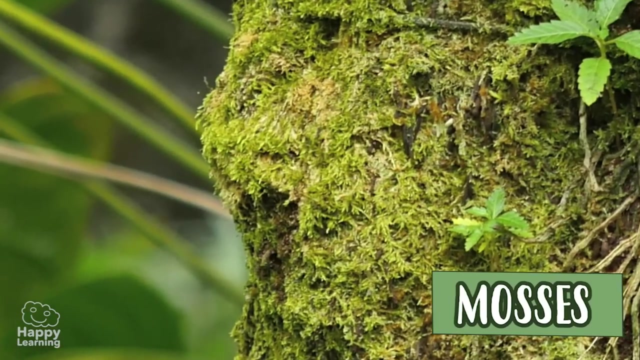 know them better. I'll guy mosses, ferns and for no grams I'll guy don't have roots, stems or leaves. they live in water but the rivers and seas and they are the simplest plants. mosses are also very simple plants. they live on solid ground but need a lot of humidity. 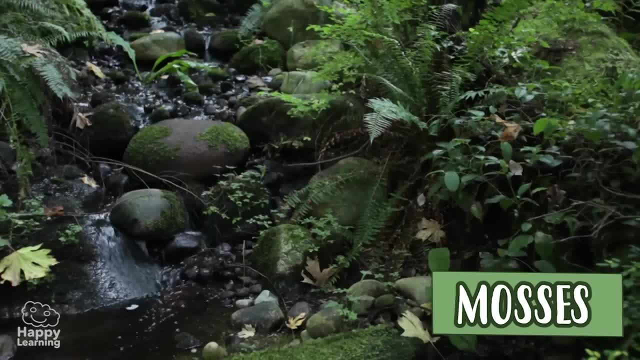 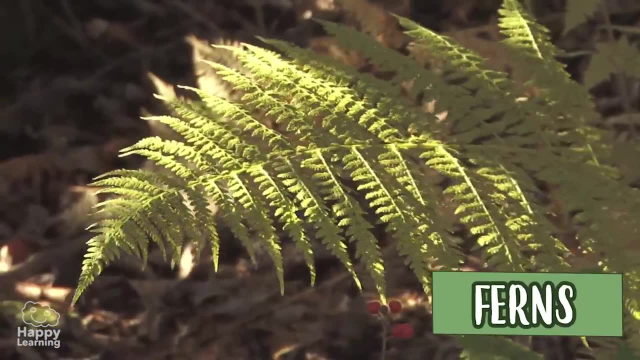 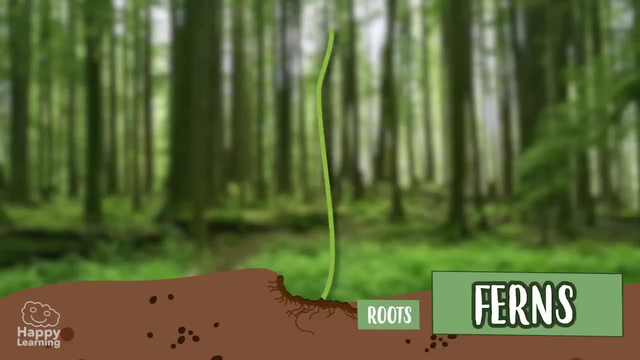 they don't have roots to absorb water because they live in very humid and bleak places. ferns are higher plants and their body is divided into roots, which is where they absorb water, from the soil stem, which is where the water circulates, and leaves that grow up in the soil. and the leaves that grow up in the soil. and the leaves that grow up. 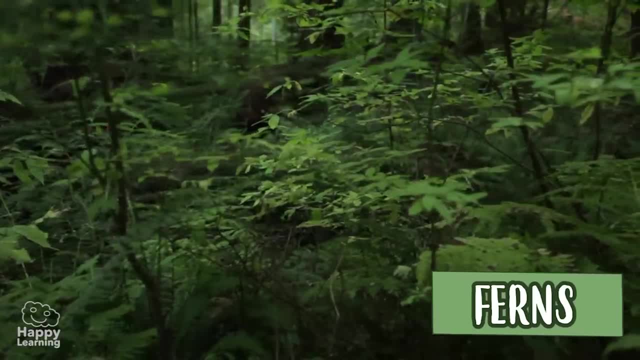 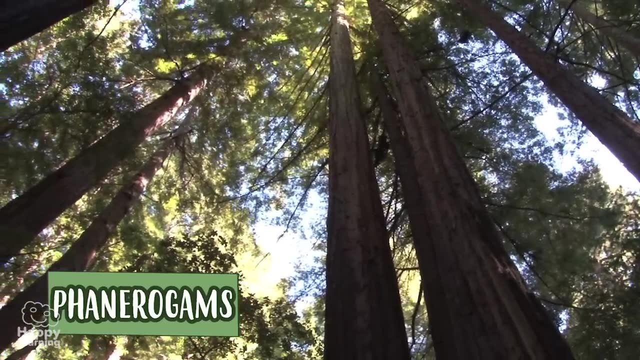 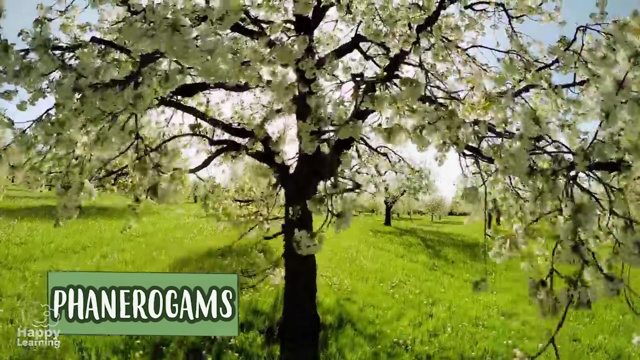 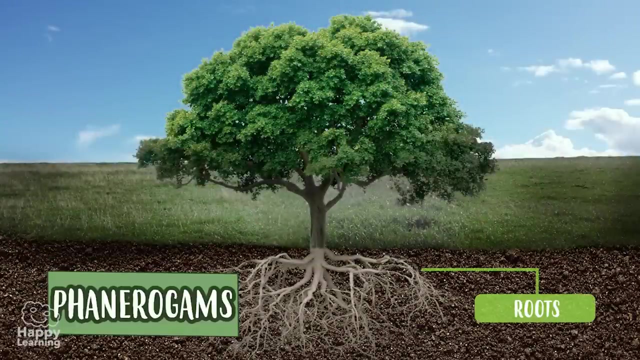 forwards from the stem. ferns also live in humid places. fennel grams, despite their name, are the most common plants because they reproduce through their flowers. they are higher plants and their bodies are divided into roots, stem and leaves. trees are an example that belongs to their school. 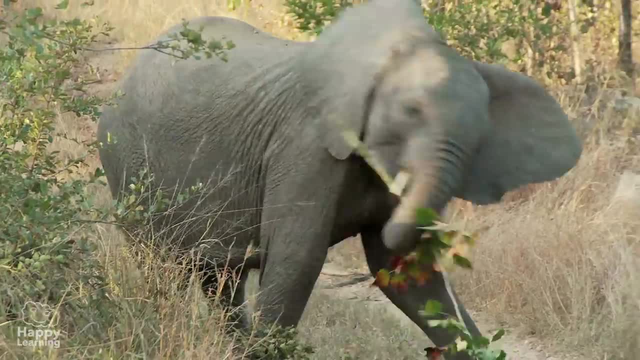 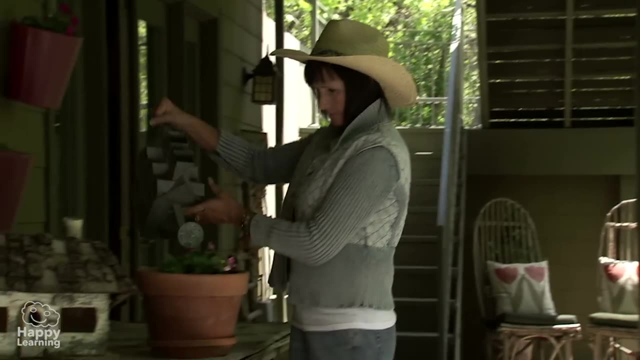 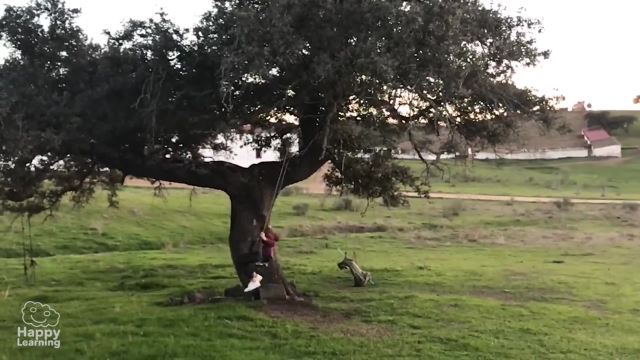 well, now we know a bit more about plants and their importance towards all other living things, so you know that we need to take care of them and respect them. goodbye, friends, and don't forget to subscribe to happy learning TV.